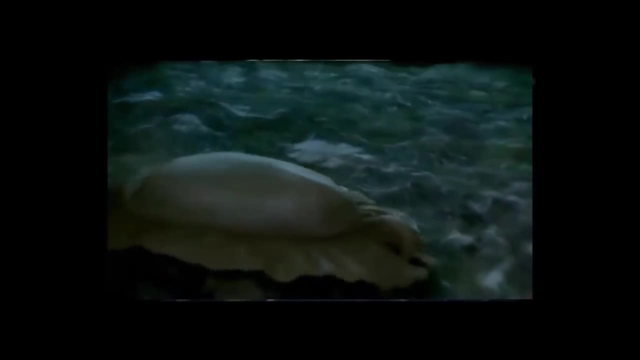 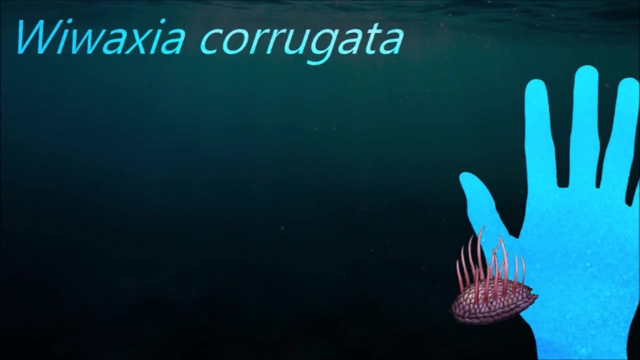 a bilaterian but not a mollusk. its age would indicate that animals were diversifying well before the start of the Cambrian. The long dorsal spines of the Wewaxia may have been a defense against predators. It apparently moved by contractions of a slug-like foot. 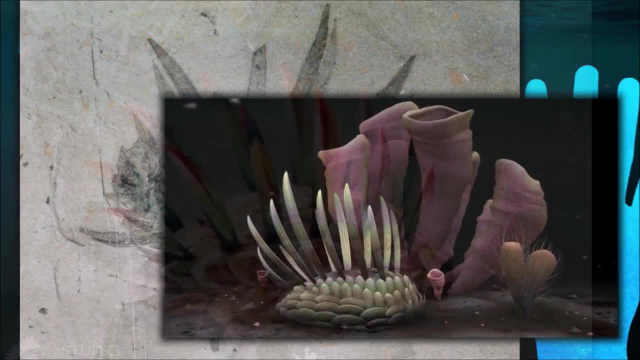 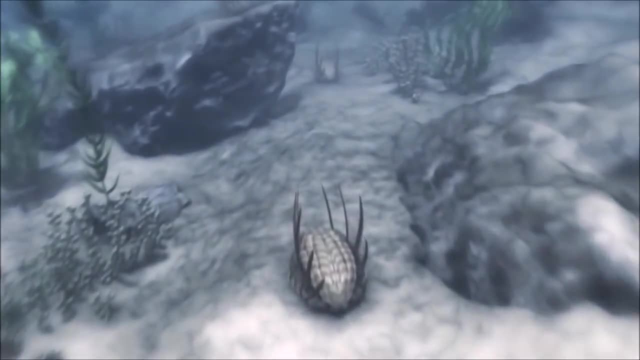 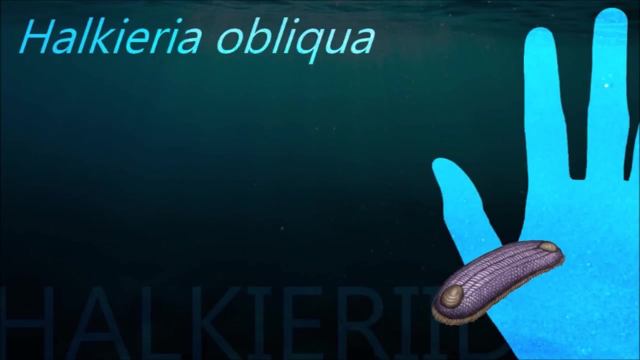 on its underside, The feeding apparatus may have acted as a rasp to scrape bacteria off the top of the microbial mat that covered the seafloor. Halkyria looked like slugs in chain mail with shell plates at the extremities of the body. 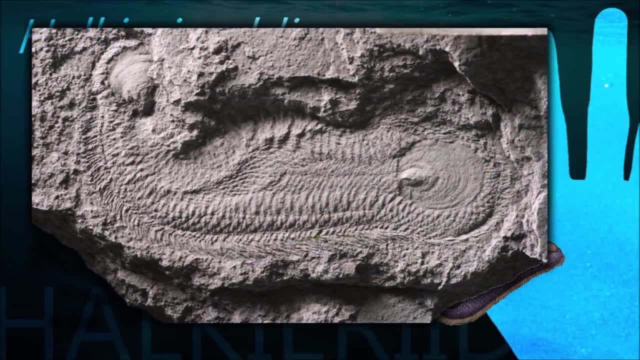 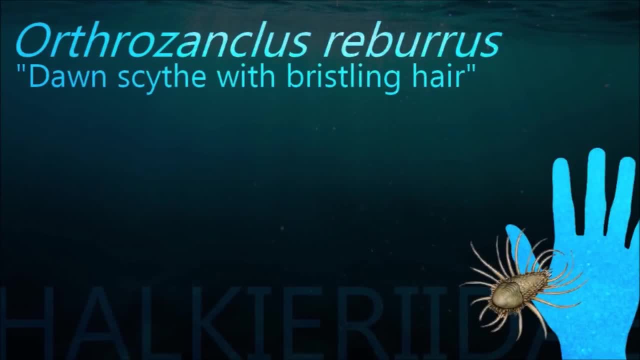 Since it was unsuited to swimming and had no obvious adaptations for burrowing, it must have lived on the seafloor walking by making its muscular sole. ripple. Orthorhynchus may have formed a link between the Halkyria and the Wewaxia. 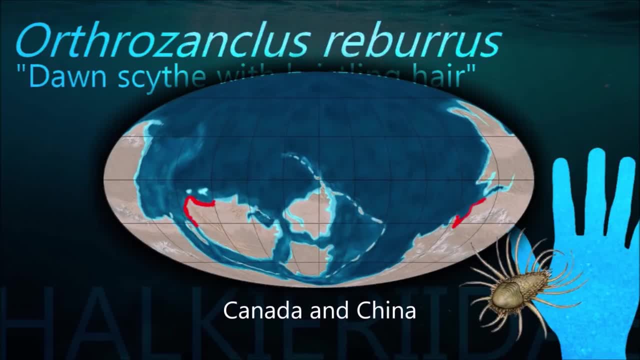 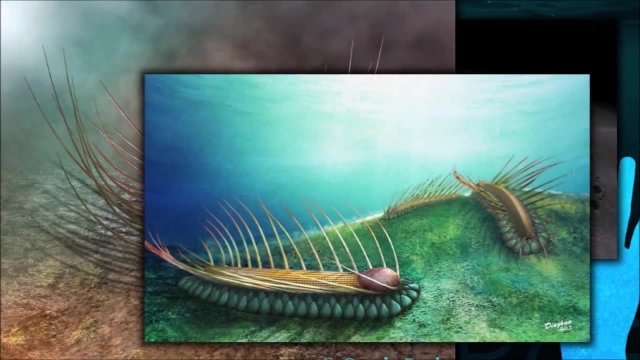 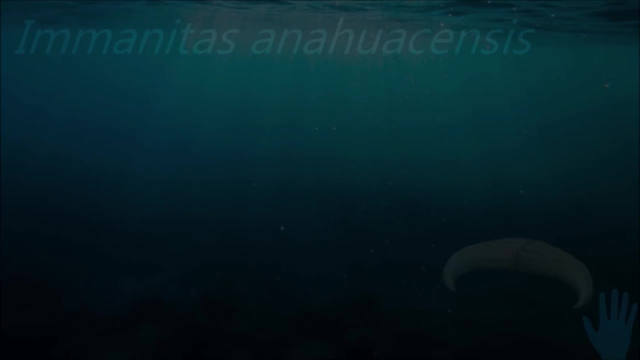 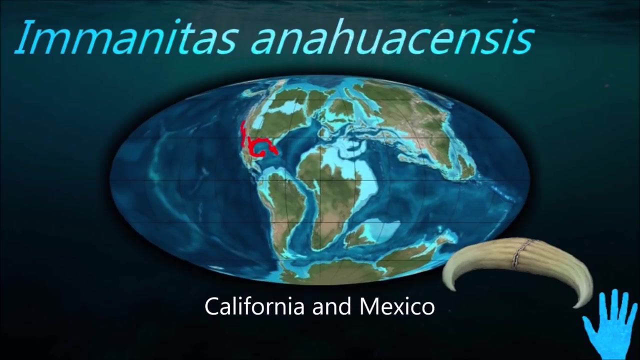 But in the Wewaxid families characterized by a similar type of body armor, these organisms might have been stem group mollusks, Bivalves as a group have no head and they lack some usual molluscan organs like the radula and the odontophore. The majority are filter feeders, The gills- 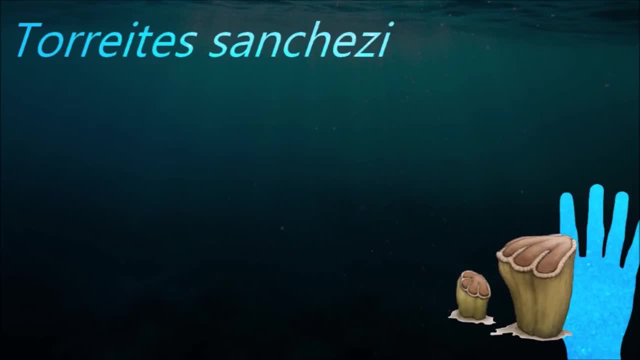 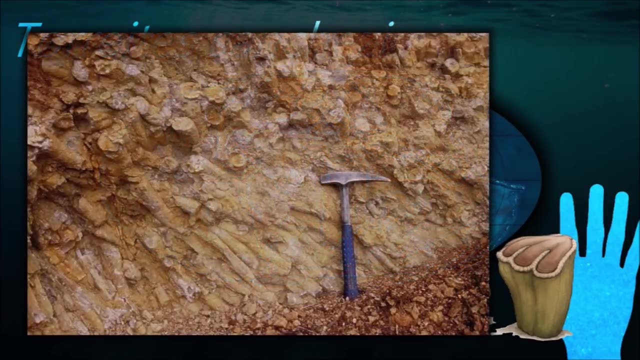 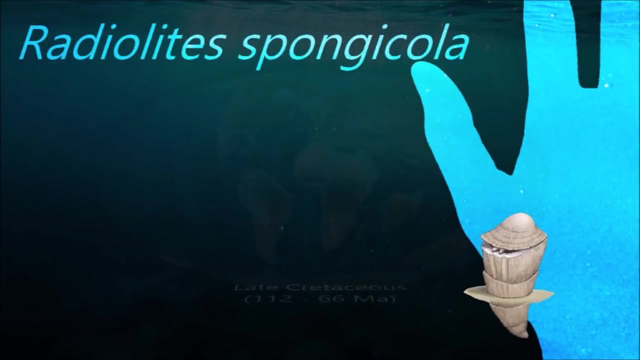 revolved in tictanidia, specialized organs for feeding and breathing. Most bivalves bury themselves in sediment where they are relatively safe from predation. The shell is composed of calcium carbonate and consists of two parts called valves. They appear in the fossil record first in the early Cambrian, more than 500 million years ago, and the total 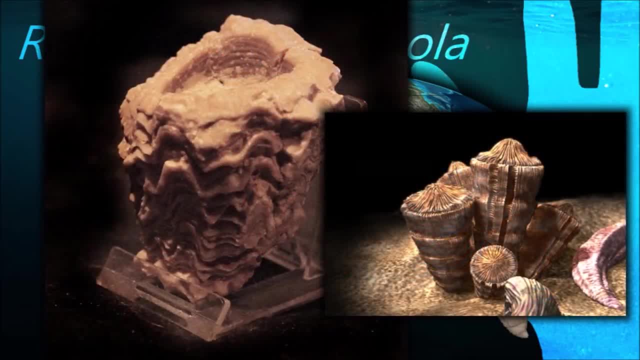 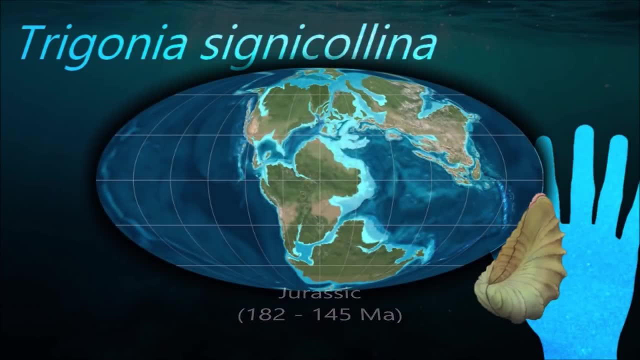 number of living species is about 9,200.. The range of the Trigone is spanned from Permian to Paleocene. In the early Cambrian's time, there were a total of 6,900 population groups, but the majority are not well-known. 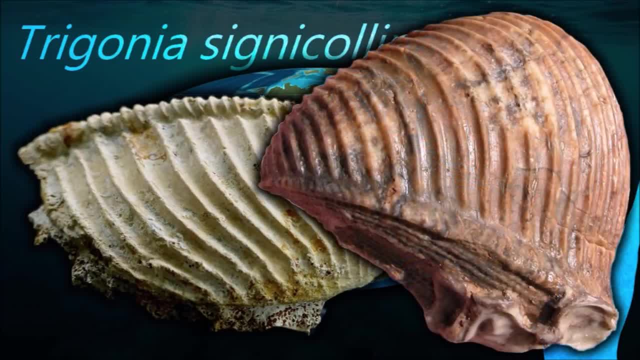 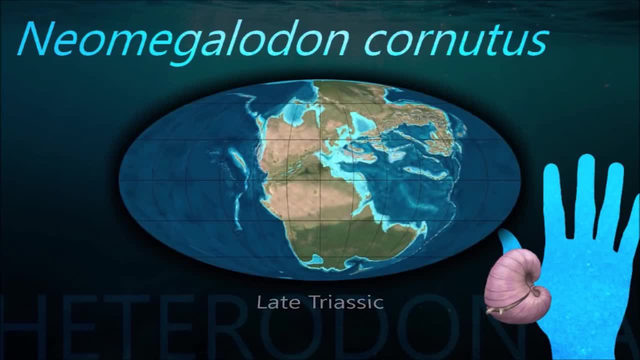 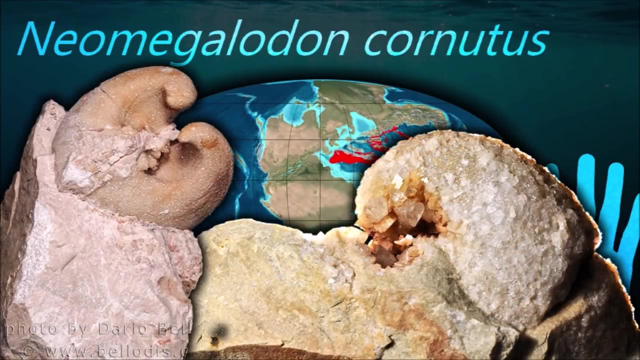 The classification of Ruddists as true Reef Builders is controversial, because they would catch and trap lots of sediment between their lower conical valves. Thus, Ruddists were not completely composed of only sand and stone. They were mainly used as sand for diceratops. 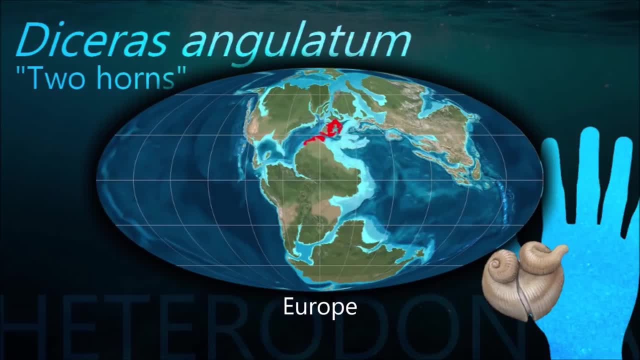 and also as a fuel for cheap water. Their manufacture was a batch of講ropolytes, a soul and a slag. In addition, sea and sea water was used as a source of oxygen levels- biogenic carbonates as a coral would be. However, rudists were one of the most important constituents. 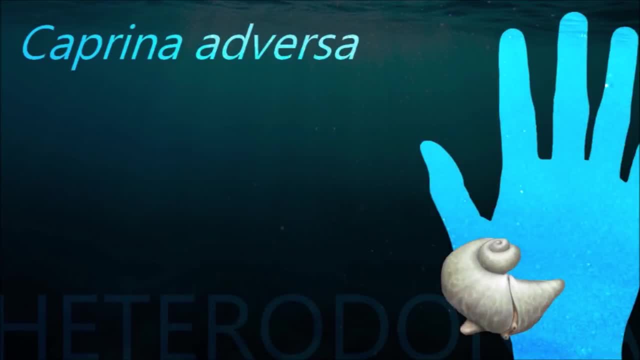 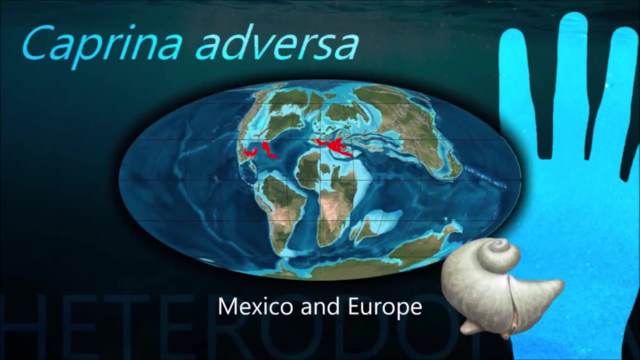 of reefs during the Cretaceous period. During the Cretaceous, rudist reefs were so successful that they drove scleractinian corals out of many tropical environments, including shells that are today the Caribbean and the Mediterranean. During this period, tropical waters were between: 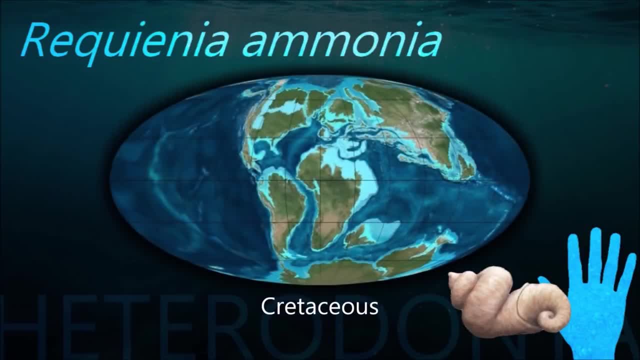 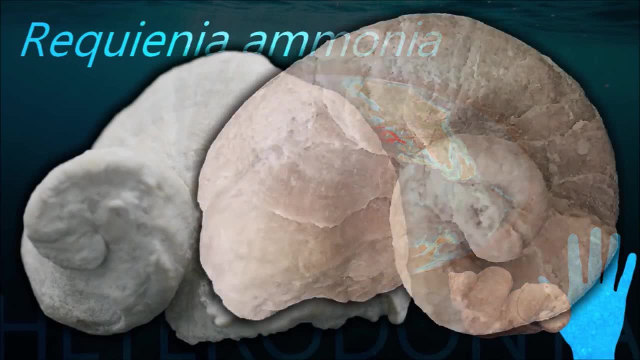 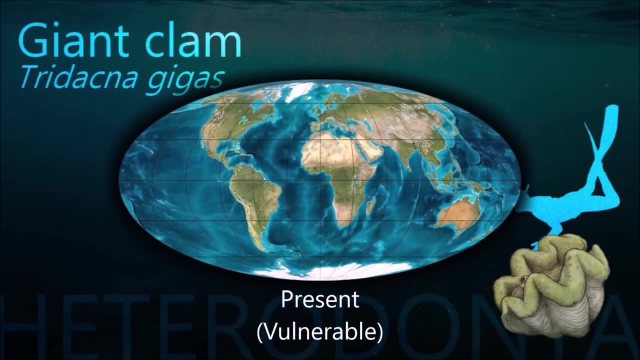 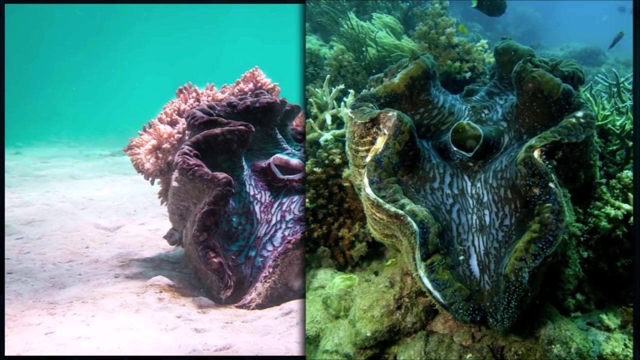 6 degrees Celsius and 14 degrees Celsius warmer than today, and also more highly saline. Giant clams is one of the most endangered clam species. their populations are diminishing quickly and the giant clam has become extinct in many areas where it was once common. They 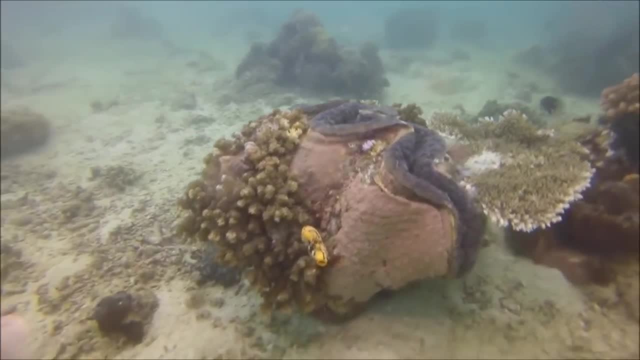 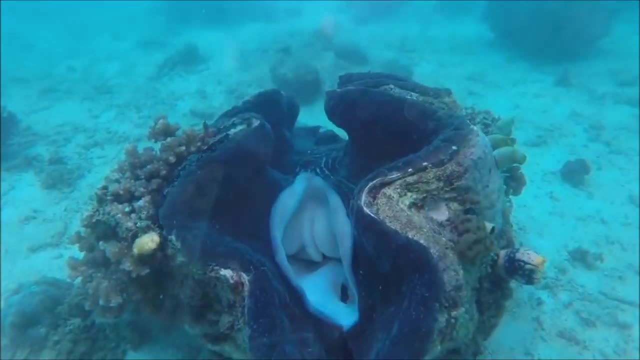 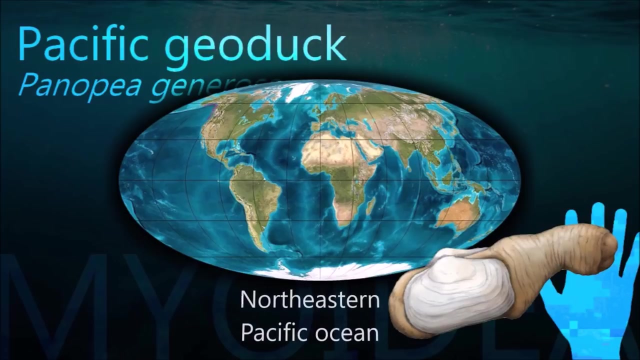 can weigh more than 200 kilograms, measure as much as 100 kilograms and weigh up to 20 centimeters across, and have an average lifespan in the wild of over 100 years. Geoducks are one of the longest living organisms in the animal kingdom, The oldest recorded. specimen was 168 years old. It sucks water containing plankton down through its long siphon, filters this for food and ejects its refuse out through a separate hole in the siphon. To escape predators such as crabs and shrimp, the flame scallops' valves are utilized. 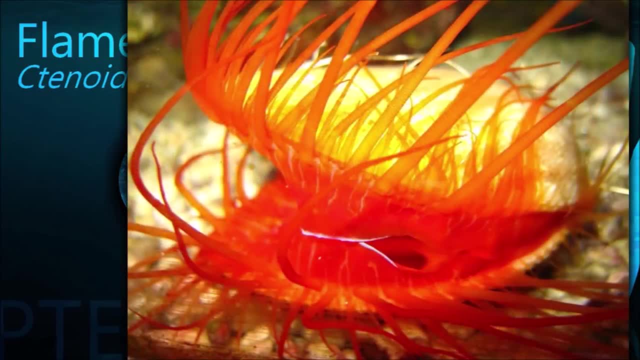 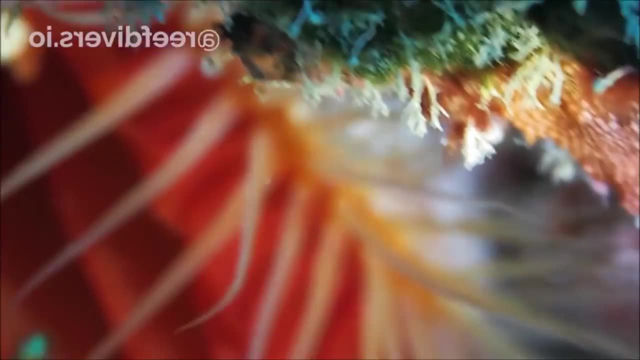 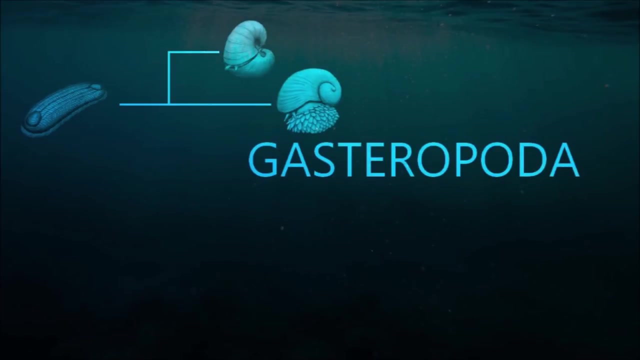 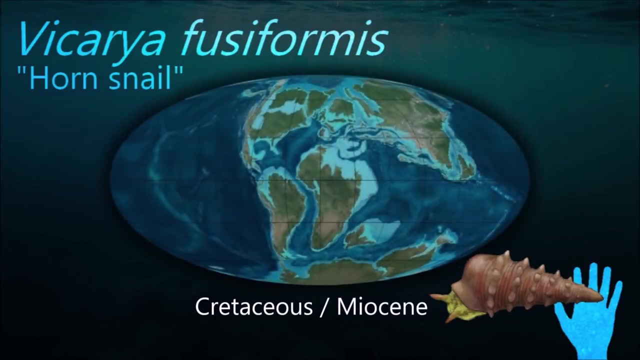 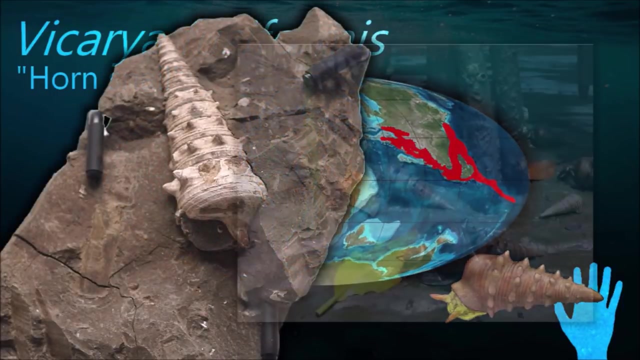 in fast locomotion, clapping their valves together to propel themselves away. Gastropoda are a major part of the phylum mollusca and are the most highly diversified class in the phylum, with 80,000 living snail and slug species. The first ones were exclusively. 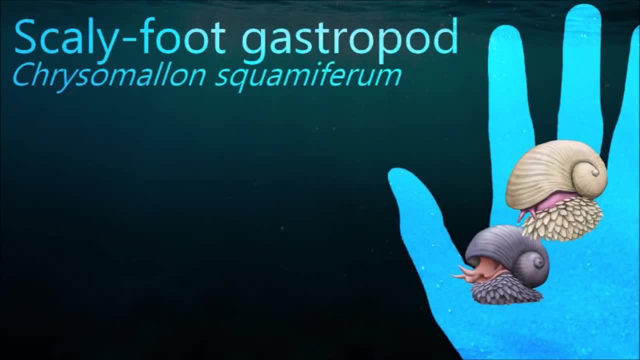 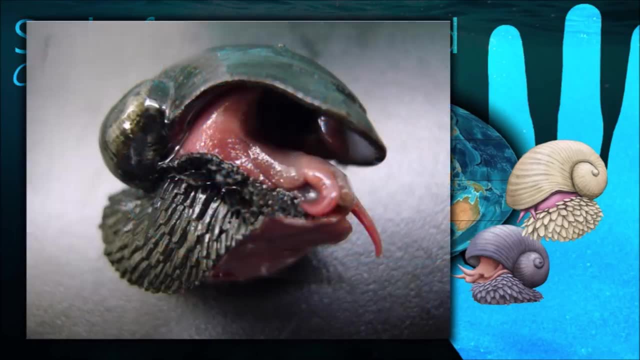 marine. The scaly-foot gastropods' esophageal gland houses symbiotic gamma proteobacteria from which the snail appears to obtain its nourishment. It is considered to be one of the most peculiar deep-sea hydrotherms. The scaly-foot gastropods' esophageal gland houses symbiotic gamma proteobacteria from which the snail appears to obtain its nourishment. It is considered to be one of the most peculiar deep-sea hydrotherms. 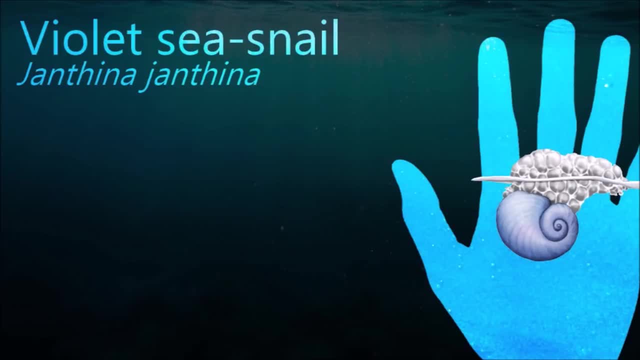 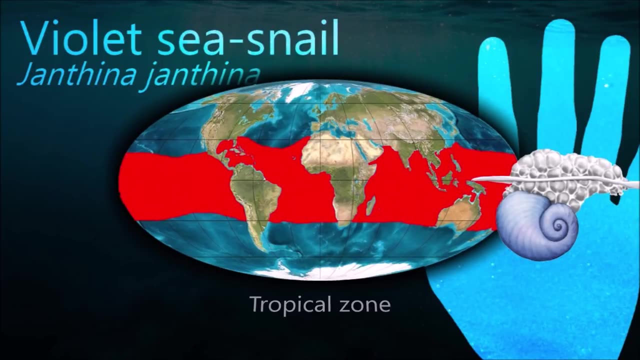 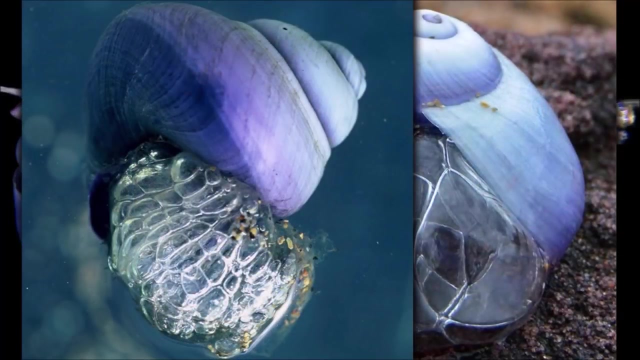 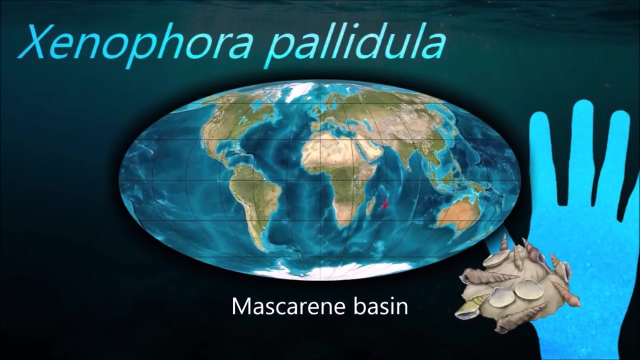 The scaly-foot gastropods' esophageal gland houses symbiotic gamma proteobacteria, from which the snail appears to obtain its nourishment. The pet- feathers, combined with its wanted fur, are the most time-consuming faculty and the skills in